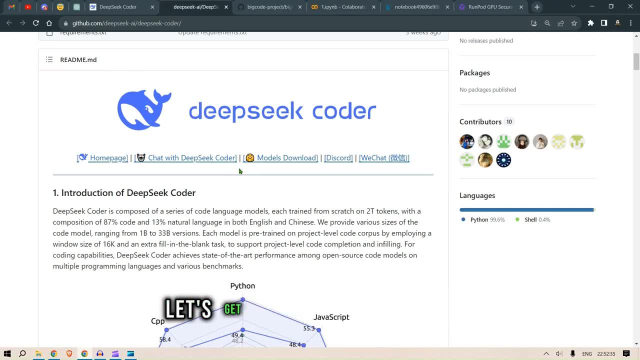 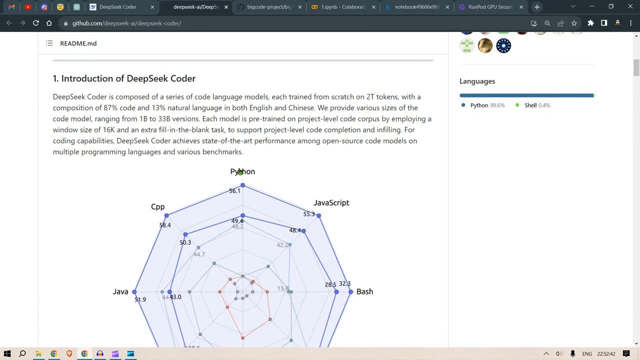 code a model for ourselves and make a model for ourselves let's get started with this video so deep this is a model it has been trained from scratch on two trillion tokens or thousand 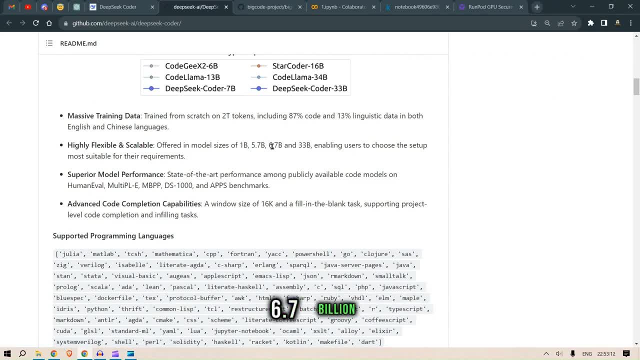 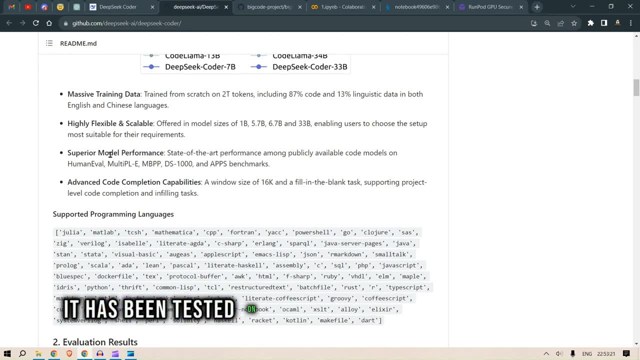 1 billion 5.7 billion 6.7 billion and 33 billion and it has been uh super it has been tested on different available code models state of the arts or soda performance on different benchmarks 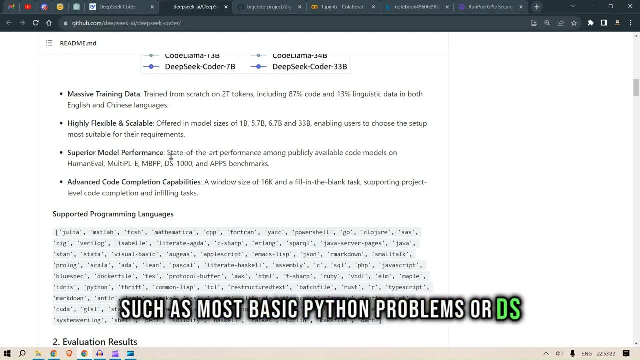 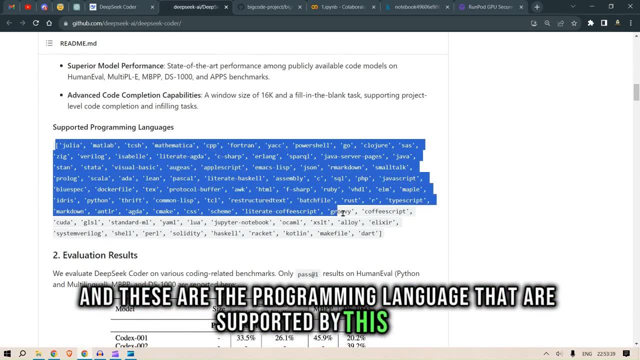 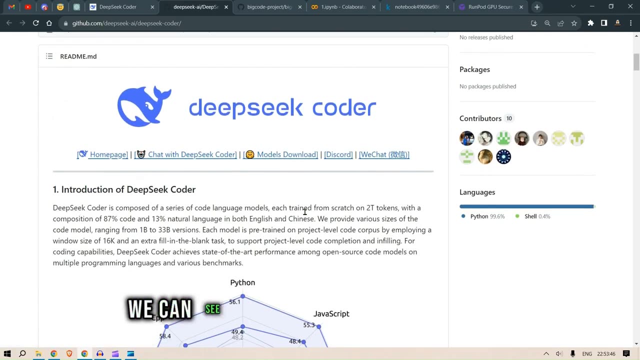 such as most basic python problems or ds 1000 apps and these are the models that are supported by this llm now we're going to look at the evaluation models but before that we can see here 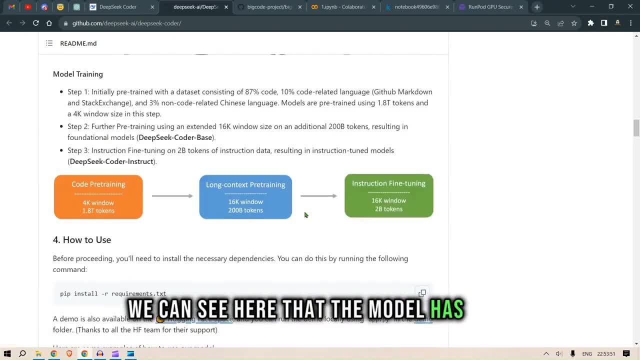 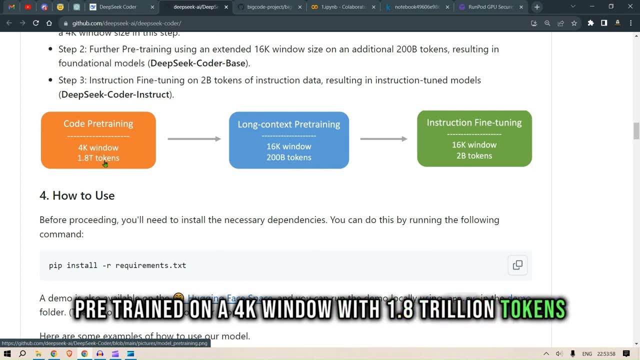 that the model has been pre-trained on a 4k window with 1.8 trillion tokens and then with the 16k window it has been trained on 200 billion tokens that is a long context pre-training 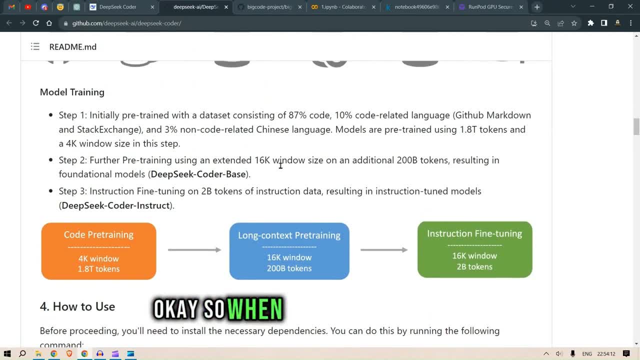 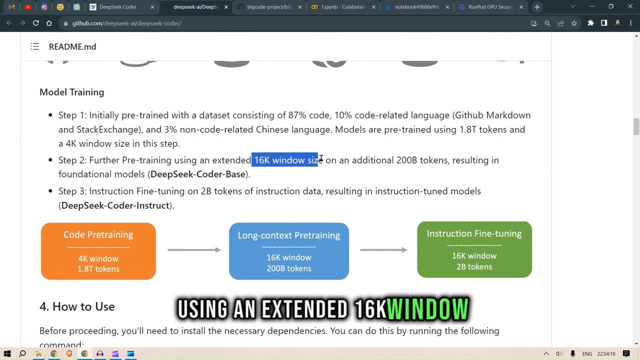 and then we have the base model here okay so when uh it is initially trained and after that when it is pre-trained again using an extended 16k window and an additional of 200 billion tokens 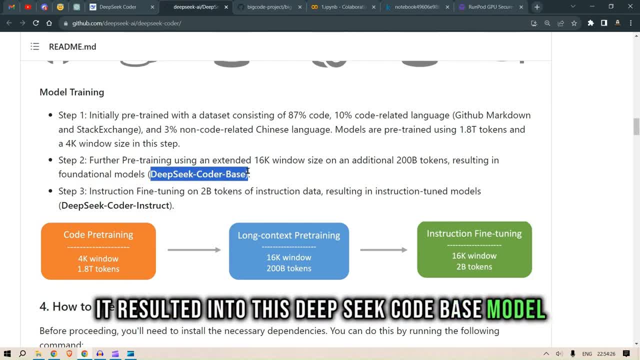 it resulted into this deep sea code base model but a base model is not strong enough to are smart enough or you know it's not it cannot reply in the format of an instruction so when you 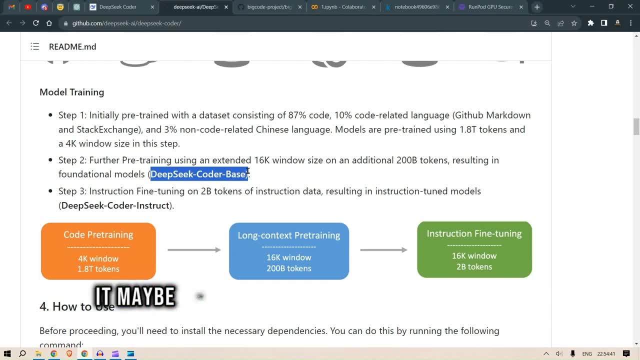 ask a question uh it replies back it maybe will reply back with the same type of question so when you say what is the color of an orange it may reply back what is the color of an apple okay 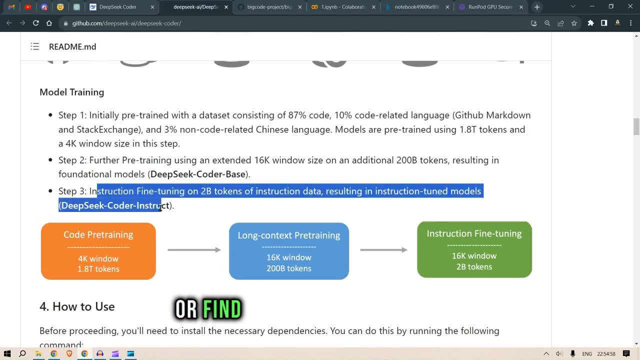 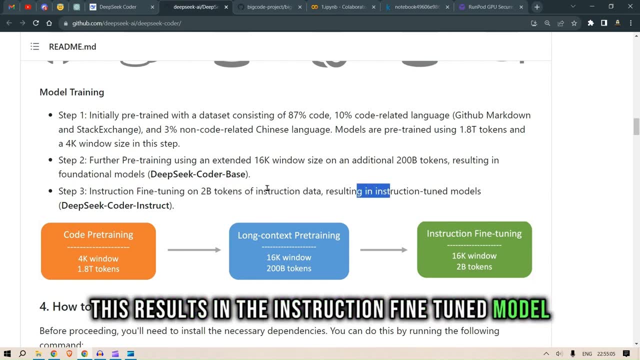 but when we fine-tune with the instruction uh tuning or fine-tuned instructions on 2 billion tokens of instruction data this results in the instruction fine-tune model it is the same way in 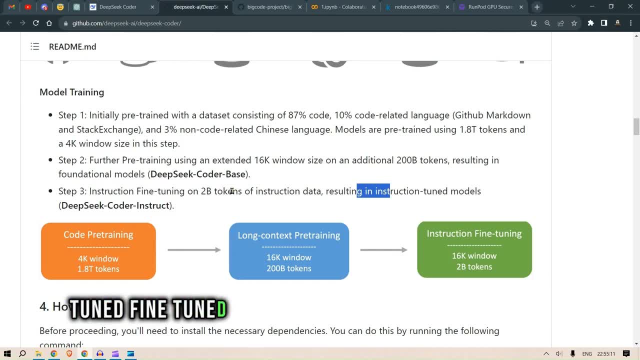 3 has been instruction tuned fine-tuned to make it into chat gpt as we know so this is the deep 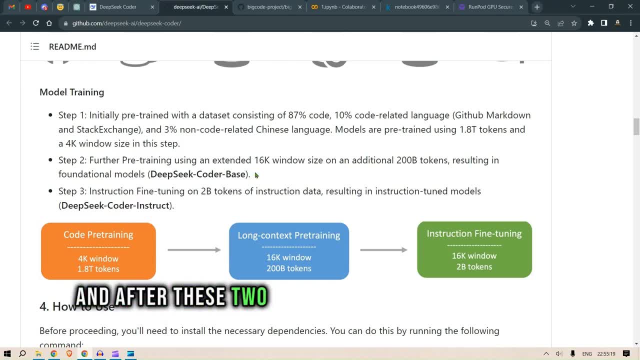 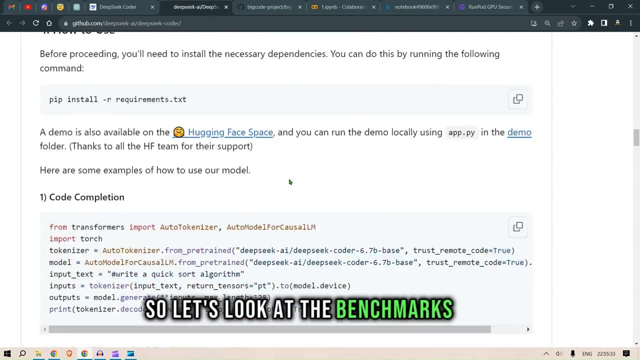 sea coder instruct and after these two steps we have deep sea coder base so i'm gonna give it a short name so dsc which is deep sea coder so dsc base and dsa instruct so let's look at the benchmarks now uh where are the benchmarks 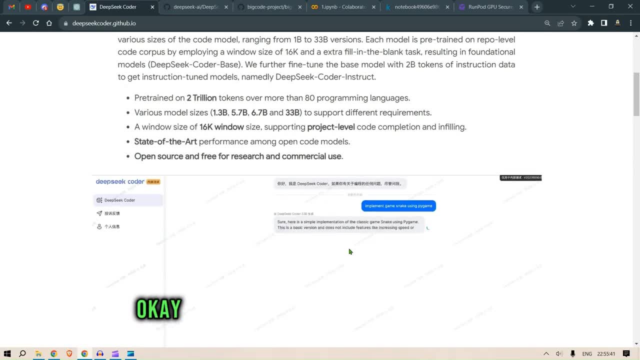 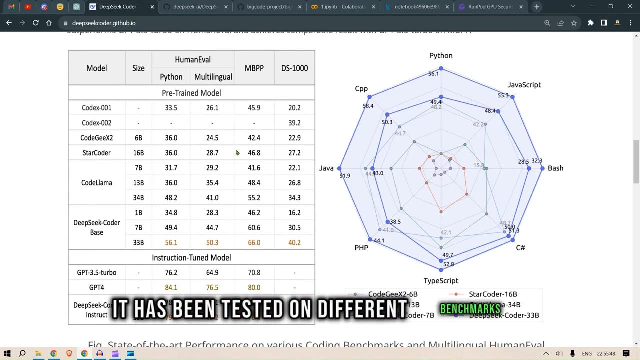 it is somewhere here okay here let's look at the benchmark uh we can see here it has been tested on different benchmarks so we have the pre-trained model here 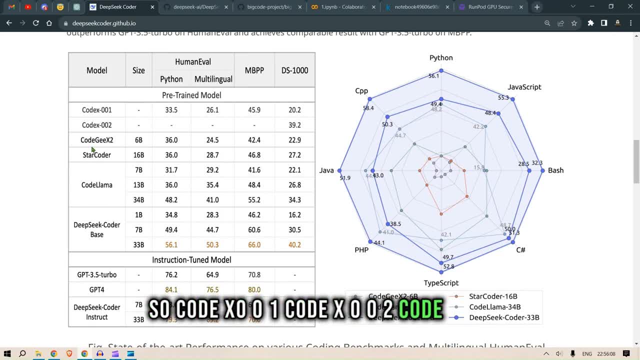 so codec zero zero one codec zero zero two code g x2 then we have uh star coder code 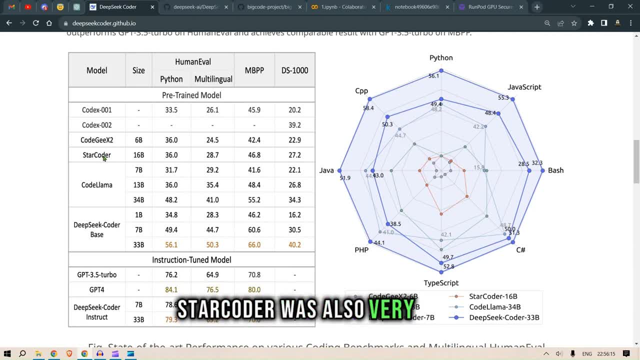 lama this was very good star coder was also very good but now we have the dsc base so in the dsc base we can see 1 billion 7 billion 33 billion and we can see the performance of you can see 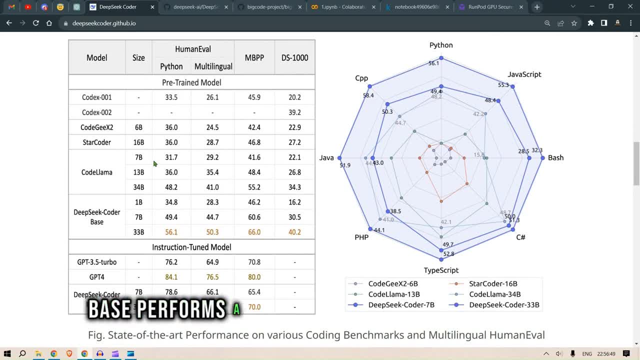 that in the dsc base performs a score of 56.1 which is very good among the pre-trained models 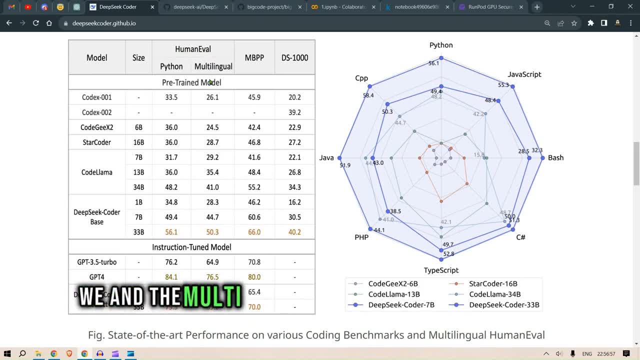 for python and human evolve we and the multilingual we have 50.3 scores very good 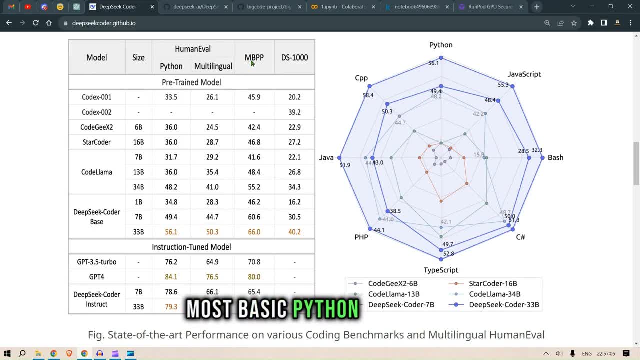 better than all the models here most basic python uh problems we have the score of this overall you 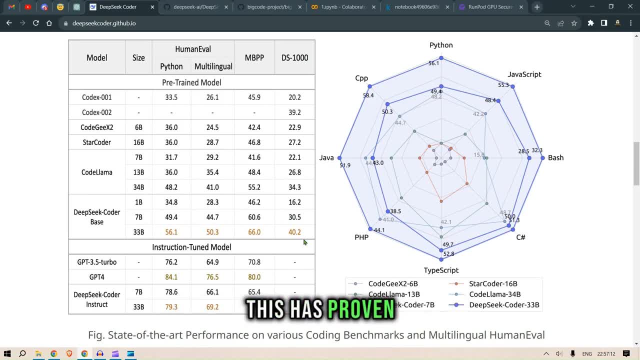 can see we have the dsc base and dsc dsc 1000 overall this has proven to be a very good 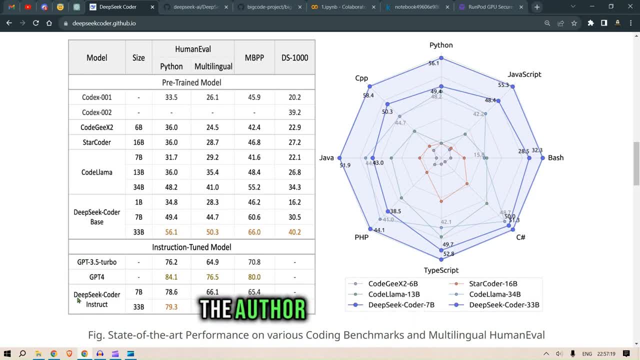 coder model below we have the instruction tune models so instruction tools the author has very 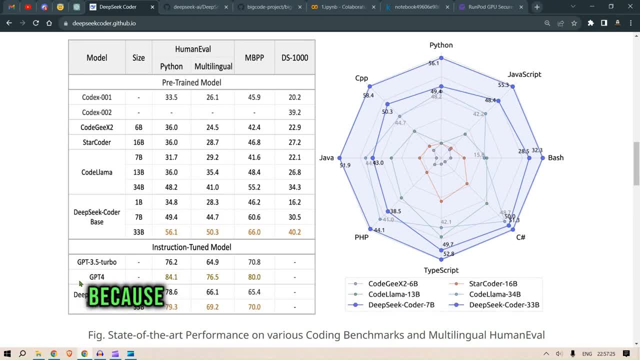 well compared with gpt 3.5 turbo and gpt 4 because these are the models that i really care about so dsc instruct it performs at par or even better with when compared with gpt 3.5 turbo 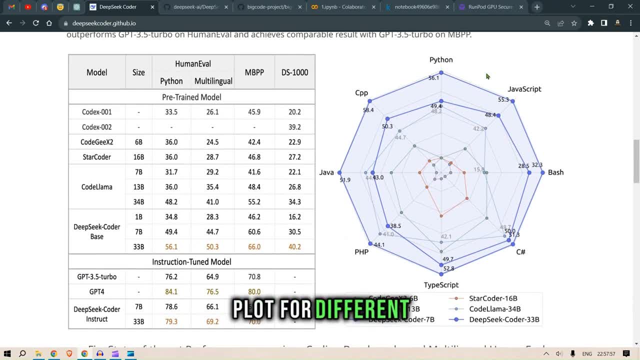 the right we have the plot for different uh programming languages here so we can see the dsc 33 billion it can perform well for all the programming languages here next uh we see the 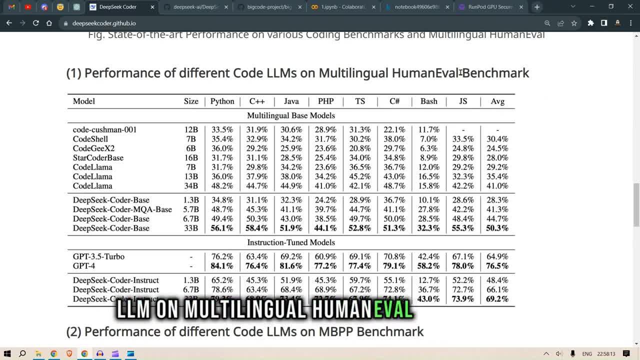 performance of different codes llm on multilingual human evolve benchmark so in this benchmark we can see that there are different kinds of uh programming languages here and we have the multilingual base models here we can see that dsc base 33 billion parameter performs very well 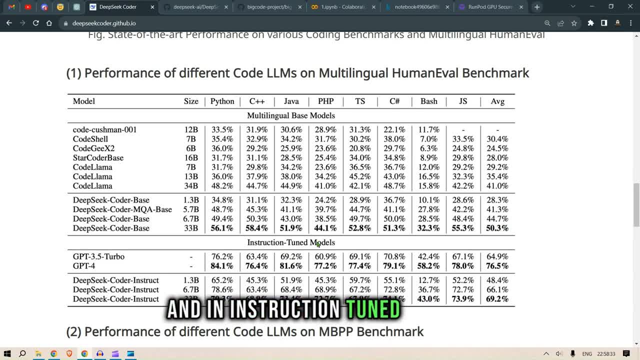 in all the languages and in instruction tune models it performs at par with gpt 3.5 turbo but it is still not able to uh compare with gpt4 gpt4 is actually very good 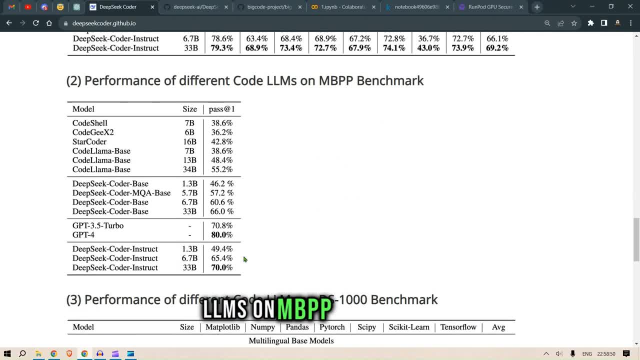 now this is the performance of different code llms on mbpp benchmark which is 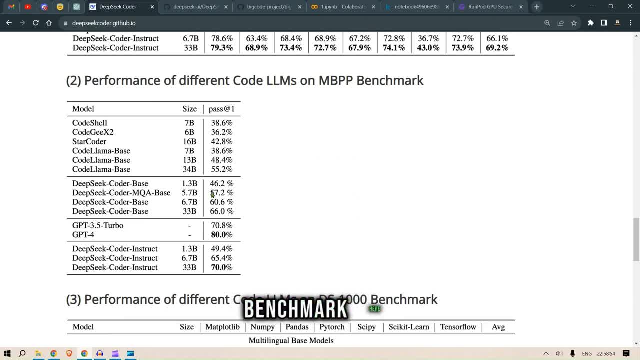 most basic python problems benchmark here also uh we have a good score for dse base 33 billion 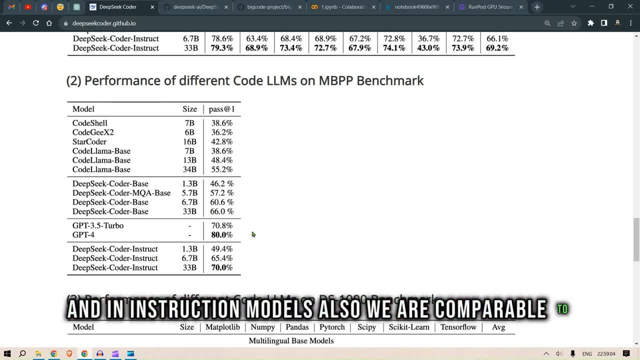 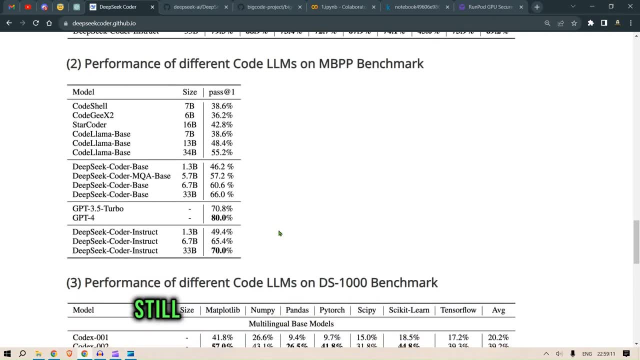 and in instruction models also we are comparable to gpt 3.5 turbo but it's lesser than gpt 4 so there is a still uh work needs to be done and maybe the next work would be done by you because 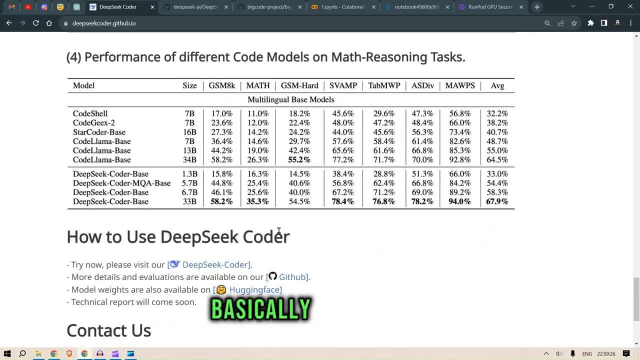 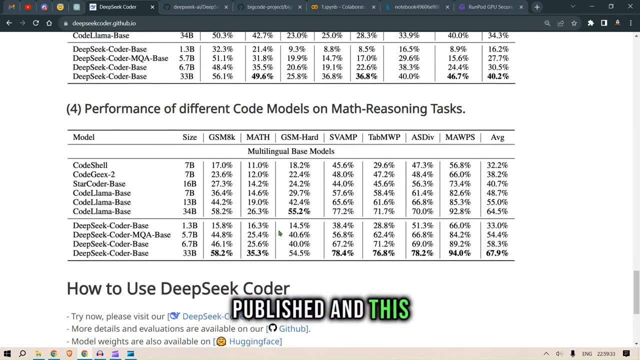 of coding so these are the different benchmarks basically it says that basically when a paper is being uh you know published and this website exists is because they're they have found some very interesting and they're able to beat a benchmark or so so here i think that it is very 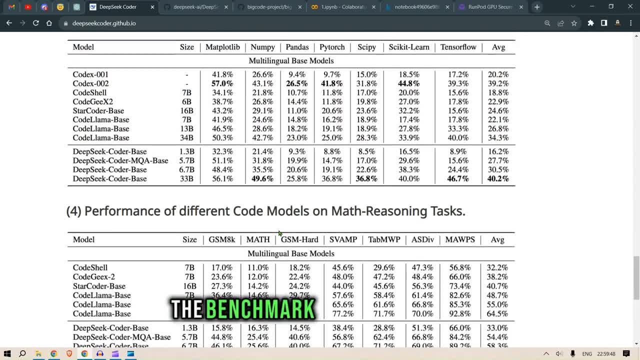 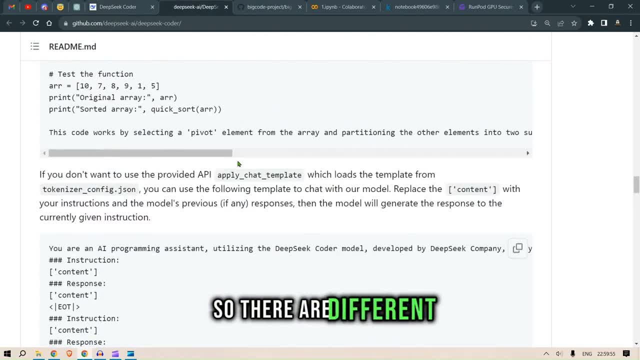 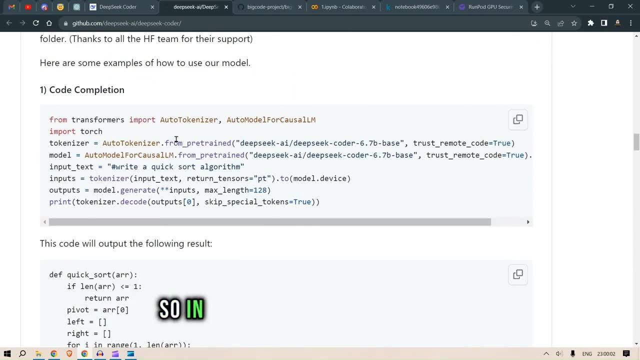 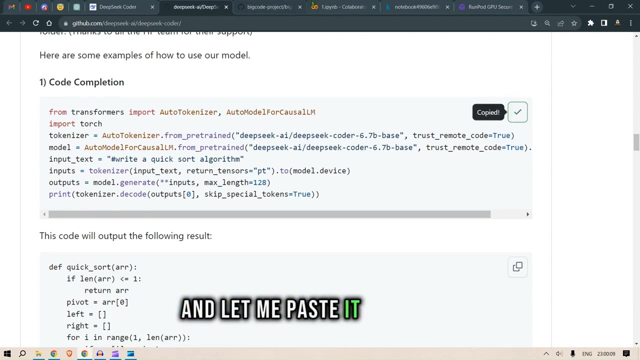 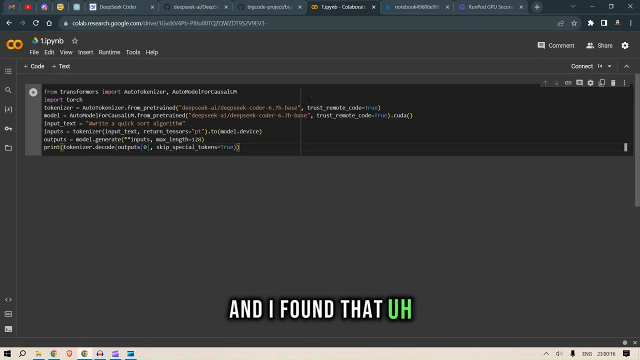 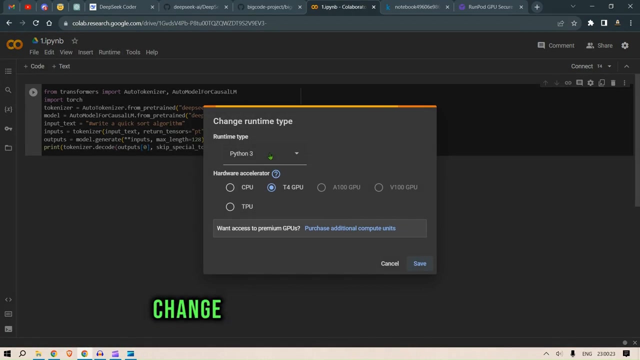 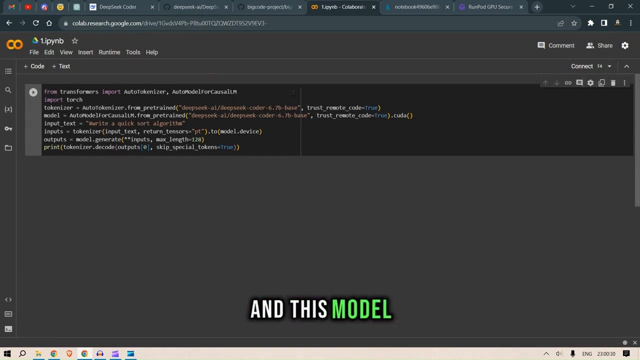 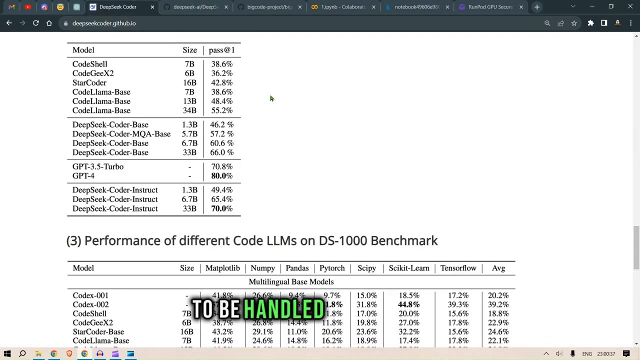 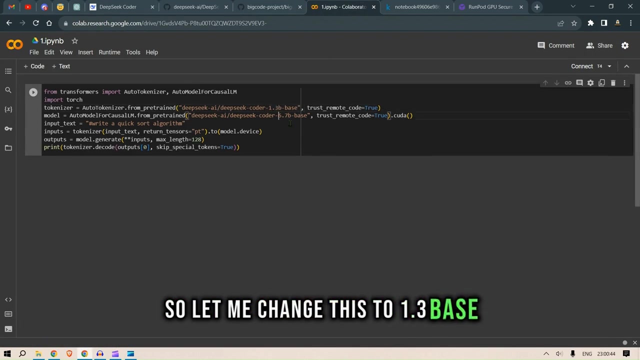 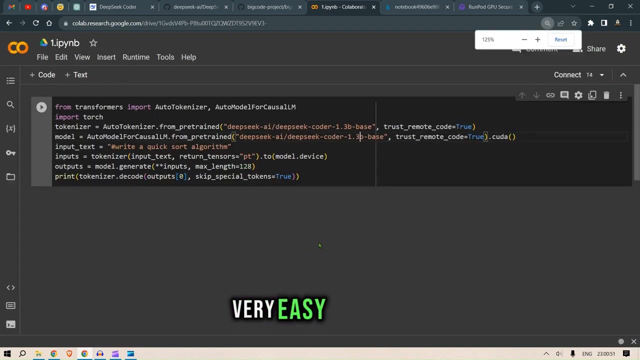 uh good that they're able to beat the benchmark of gpt 3.5 turbo now let's test it out and let's see so there are different uh types of tests that you can do the first is code completion so in the code completion we have for example from this is the code let me copy the code here and let me paste it in uh collab google collab now i have tested this out and i found that uh the memory here if you go to runtime uh disconnect here and you can change the runtime here to uh tp gpu and this uh model you know these uh three 6.7 billion parameters not uh will not be able to be handled by our collab a free collab so i need to change it to 1.3 so let me change this to 1.3 base and let me explain this code so this is a very very uh of this model so from the transformers library we import the auto tokenizer that is used for tokenizing from text to numbers and vice versa from numbers to text this is auto model for causal llm this is for starting of a model for causal inference causal is me it means predicting the next token so we are going to import torch then tokenizer we're going to start this tokenizer we're going to load the model here 1.3 billion base and then we're going to say trust remote code is true because we are running from our system here then you're going to load up the model auto model for causal uh from pre-train 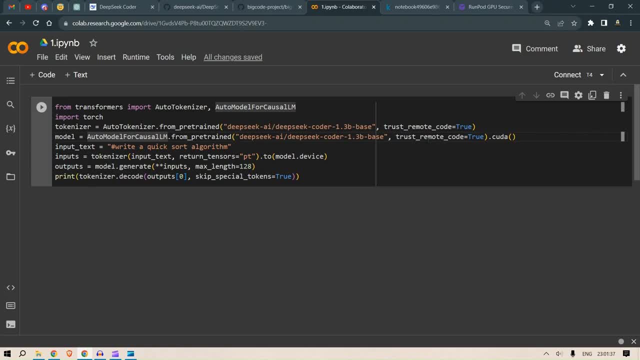 we're bring going to bring this model up and trust remote code to true and send to CUDA if available next input is write a quick sort algorithm this is our input prompt then this input is tokenized okay so we tokenize this input using this tokenizer which is an instance of auto tokenizer so tokenizer is input text we get the we return the tensors as 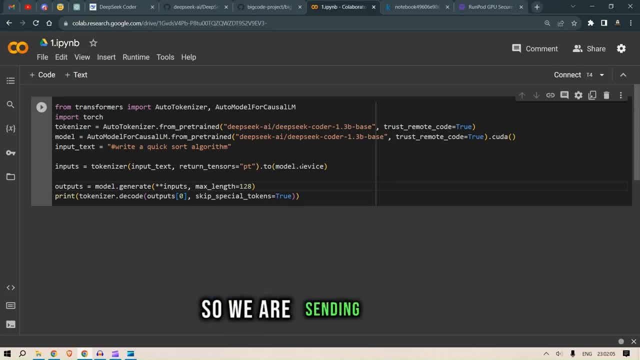 PT and we send this to the model.device so we are sending this to the same uh device that we have instantiated that is CUDA now output is just the output model.generate and put in the inputs here and we just print the tokenizer we print the latest output and we get out the results 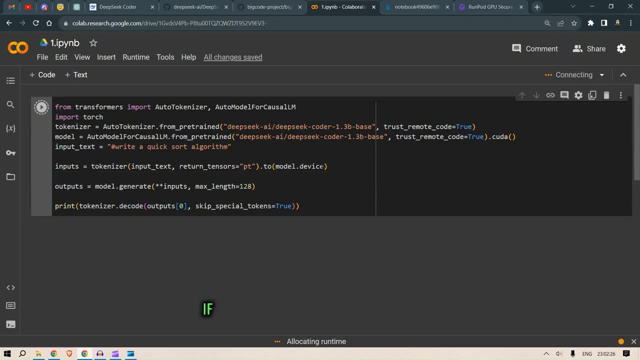 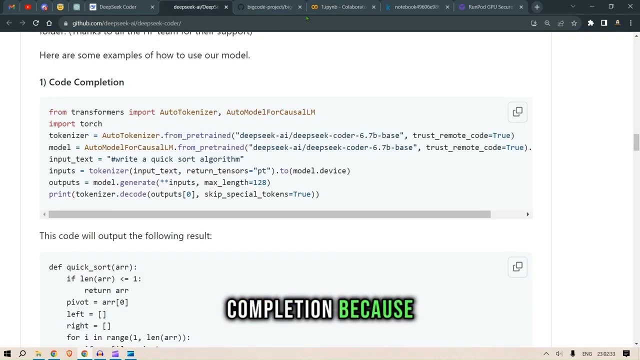 so let's run this and let's see if we are able to connect so this is uh uh you know code completion this is code completion because we just give it a prompt and it is going to complete the code here 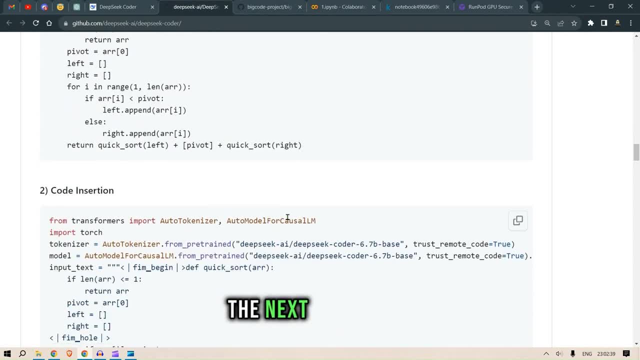 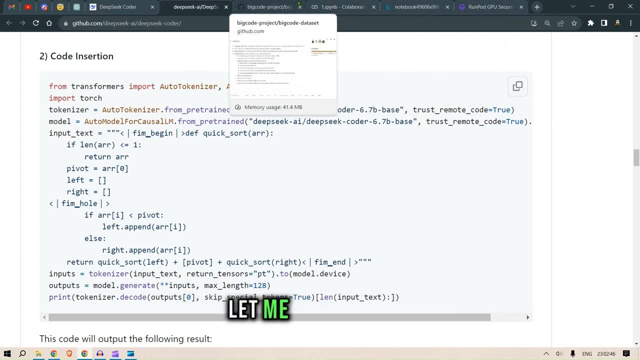 now while this is running we can look at the next uh thing that is available this is uh known as a code insertion so this is different method let me go to Kaggle notebook this time and paste it here 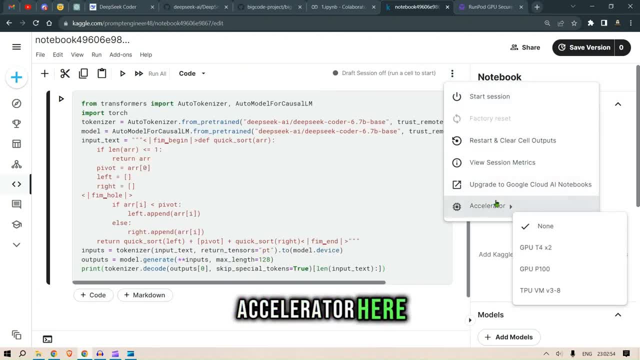 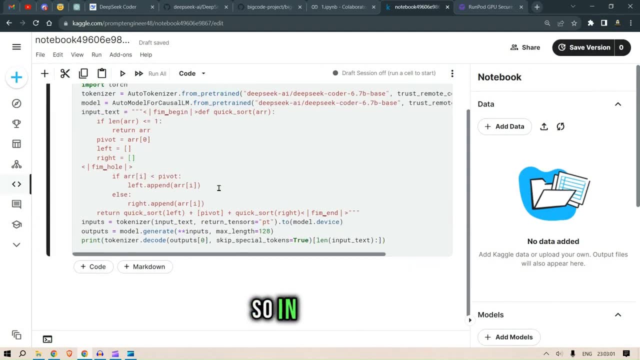 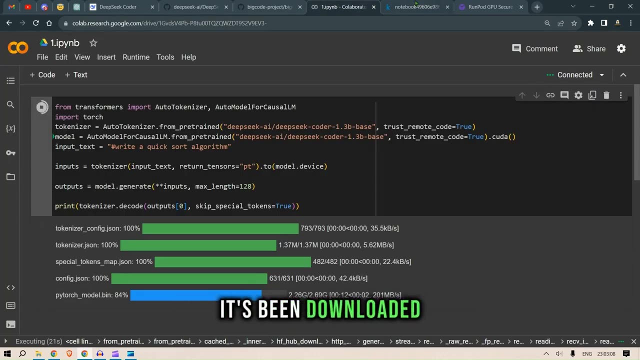 and let me select uh an accelerator here uh let's take GPU uh p 1000 p100 so in this code it's almost the same thing we import the transformers let's see the result here okay it's being downloaded 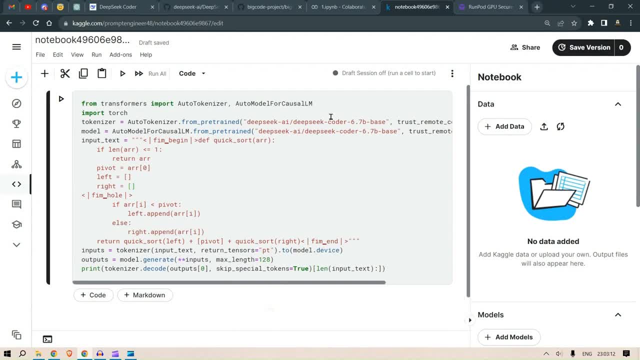 so from transformers we import the auto tokenizer and auto model for causal LM then we import the 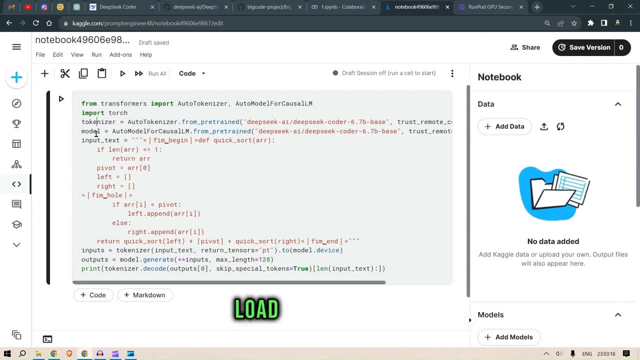 torch we start the tokenizer we load up the model and in the input text what we have is this so within three quotation marks we have this input this input is actually a part of the quick sort algorithm but 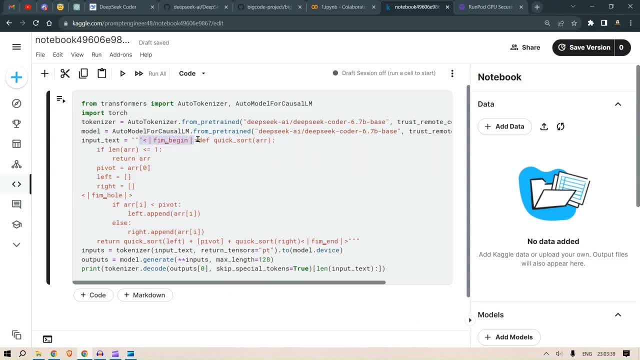 here we define the special tokens which is FIM begin and this is FIM end so these special tokens it's not like that uh you can define this tokens it has been defined by the developers who created this uh model 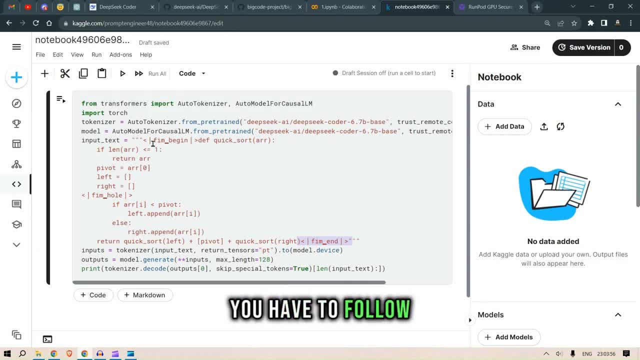 so this is strictly something that you have to follow uh these tokens so if you want to do the code insertion kind of thing you need to put in this begin end and there is this hole here FIM hole so here the the algorithm will run and will fill in the codes the missing codes in this 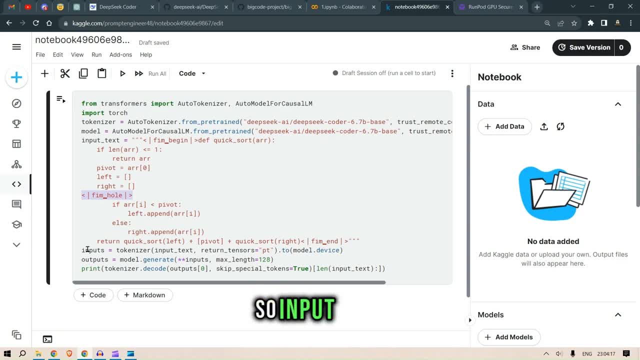 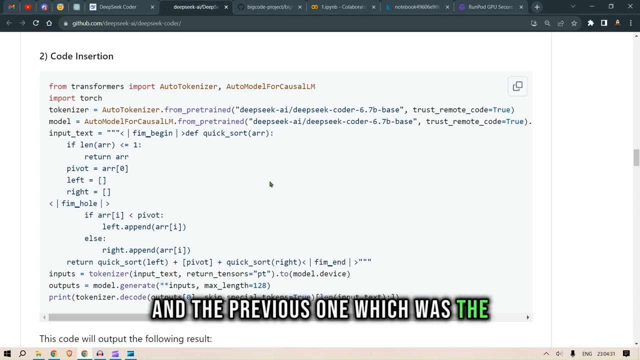 whole portion so we'll run this so input is the tokenizer uh dot input text and output is the model rate and print the tokenizer.decode so run this and the previous one which was the uh you know which 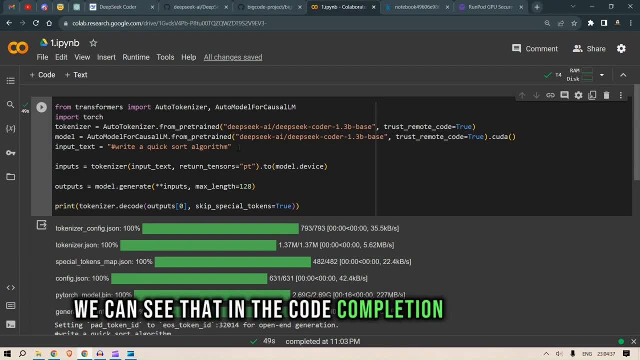 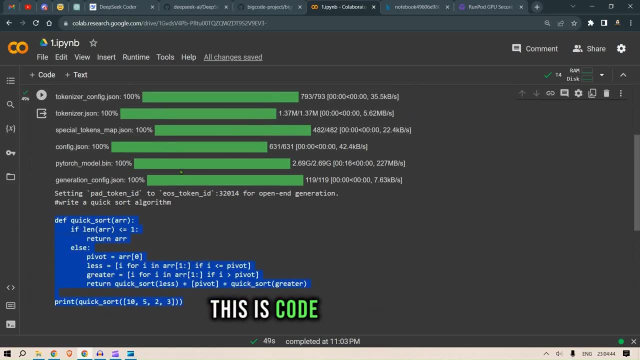 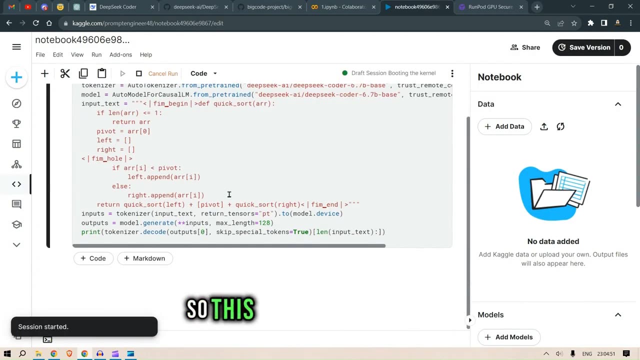 was the code completion here we can see that in the code completion we have this so this is the code completion we have this beautiful uh code being generated this is code completion next in the Kaggle notebook we are running this and the session has started so this is the code insertion 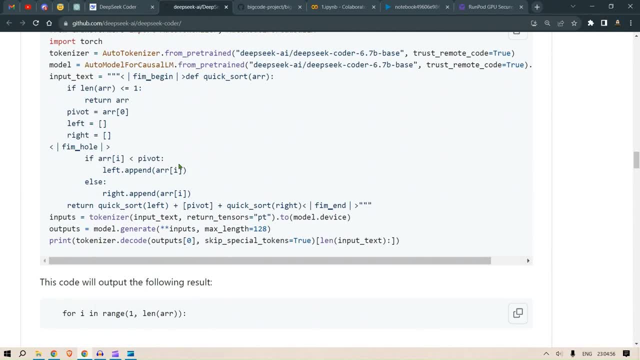 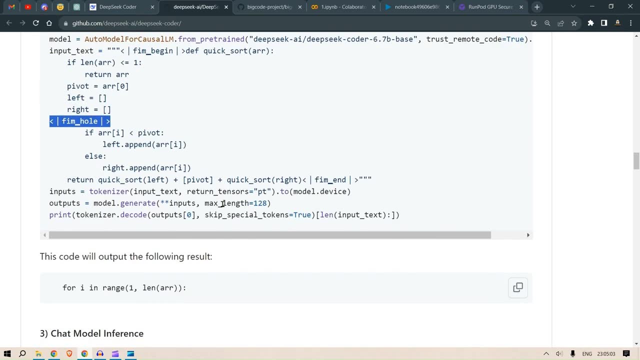 because we are going to insert the code in the in the center or somewhere within the code there is a hole being created and we are going to insert whatever the missing components are in inside in 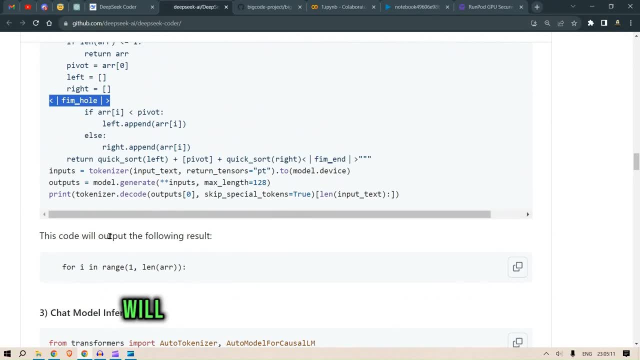 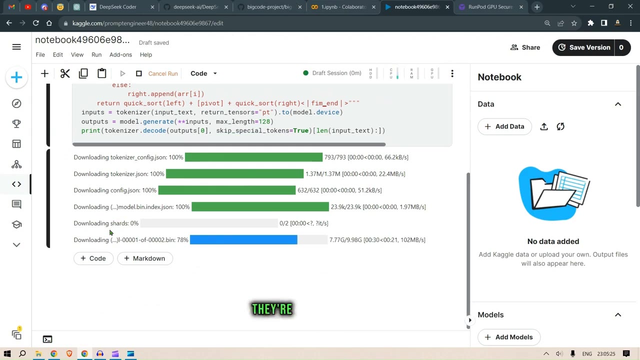 the hole in the place of the hole so the code will output the following because this is missing and this should be in the hole itself so let's wait if the code is able to generate that so it's loading here and it's loading on the shards shards you know they're different uh if you have a let's say a 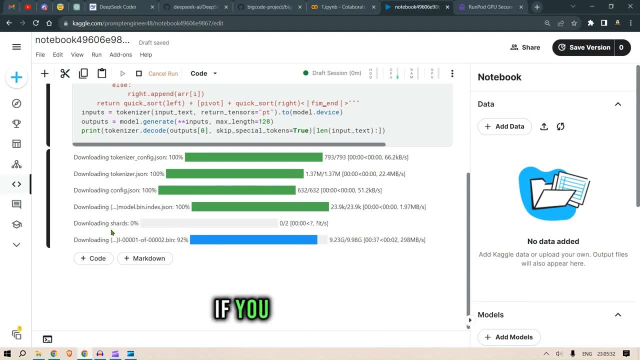 20 GB model and uh if you create four shards so five GB model uh there will be five parts four parts of five GB each so four shards now I think there should be two shards here because one is of 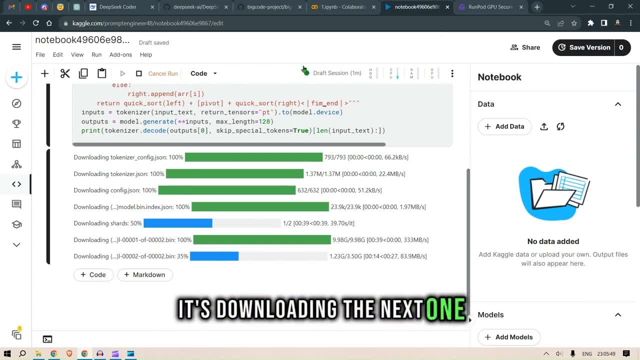 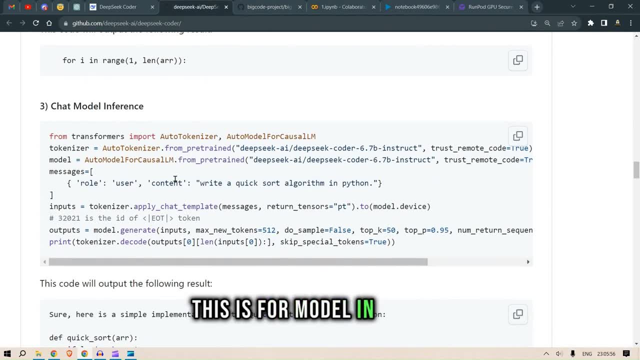 two so one of two has been downloaded it's downloading the next one but instead of waiting on to the next uh thing that you can do this is for model inference this is pretty simple it's like 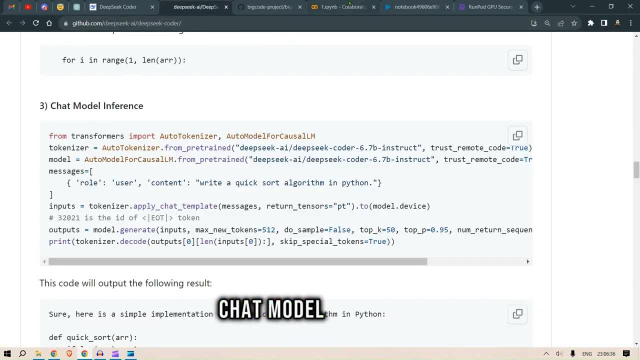 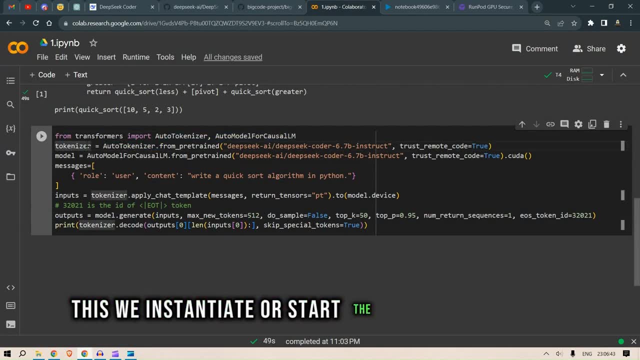 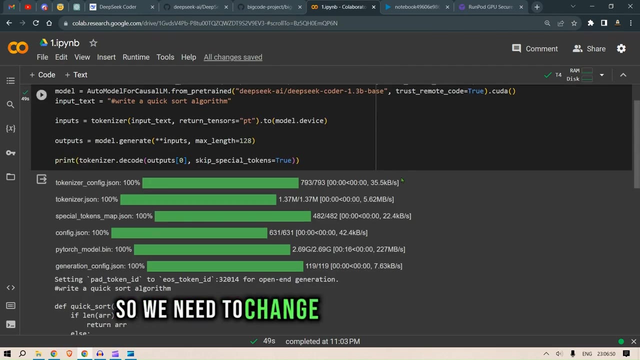 uh an instruction so we go chat model inference so from transformers we import the auto tokenizer this we instantiate I start the tokenizer using the DSC 6.7 billion instruct so we need to change 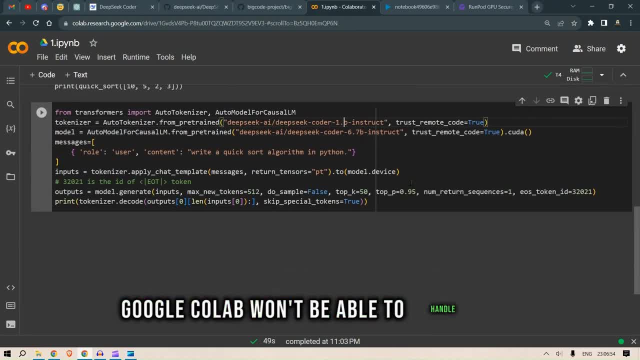 this because our free Google collab won't be able to handle this 0.3 billion instruct we load up the model here and this is the message here so role is user and 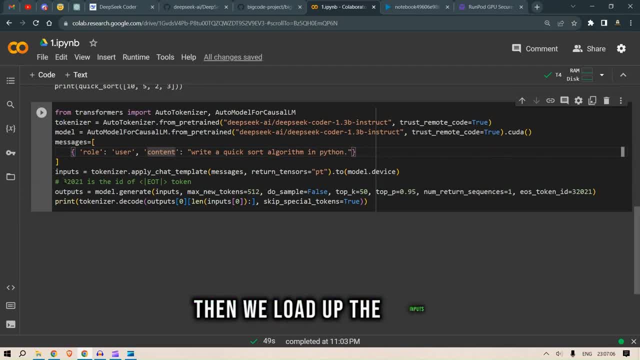 content is write a quick sort algorithm in python then we load up the inputs same as usual this is the output being generated and this is the outputs being decoded with the help of tokenizer 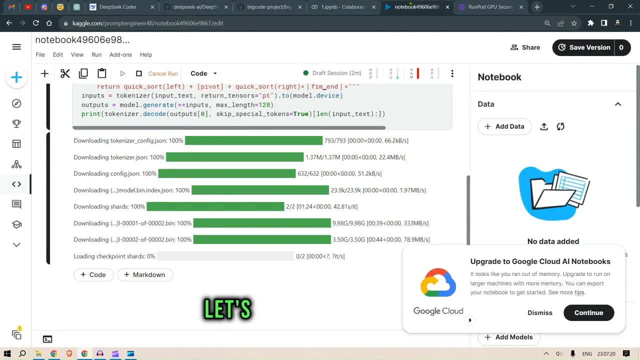 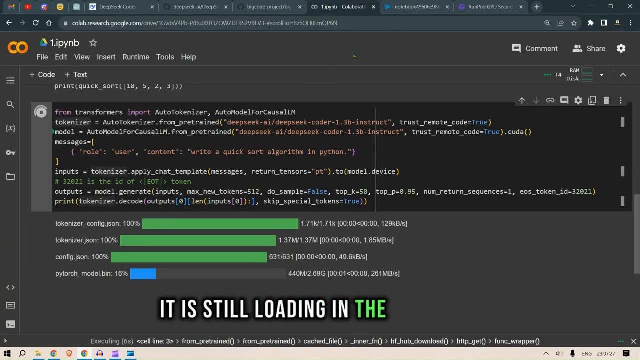 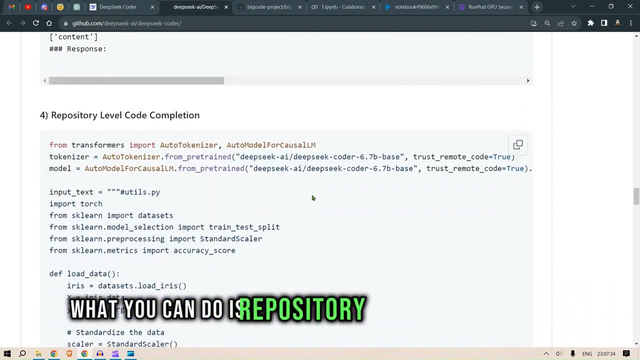 and we are just printing the output so let's run this let's go to the notebook so it is still loading in the notebook next chat model inferences this next what you can do is repository level code 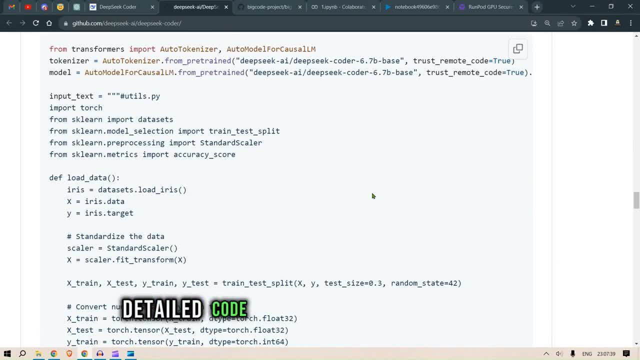 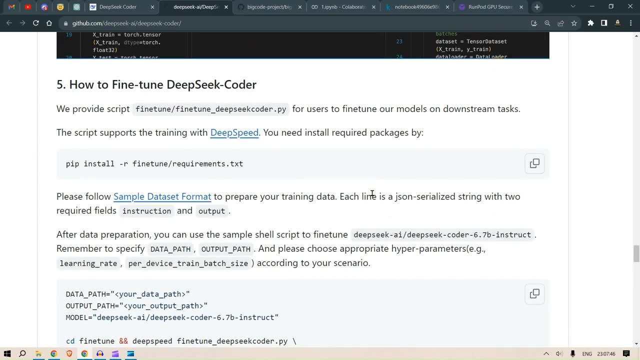 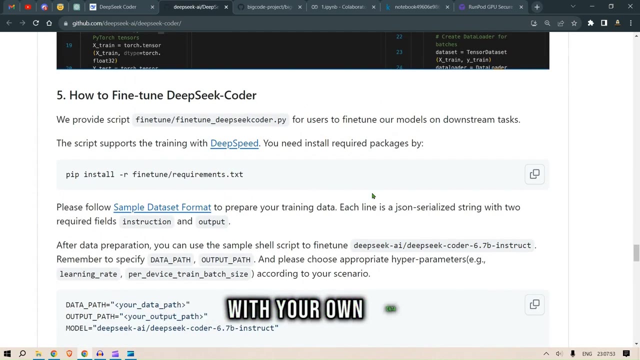 completion so this is again a very detailed code that you can have a look at now please try this out I am not going to try this out you can also fine-tune on the DSC uh with your own data but 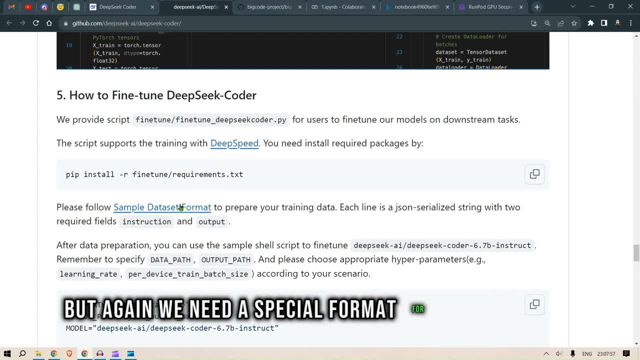 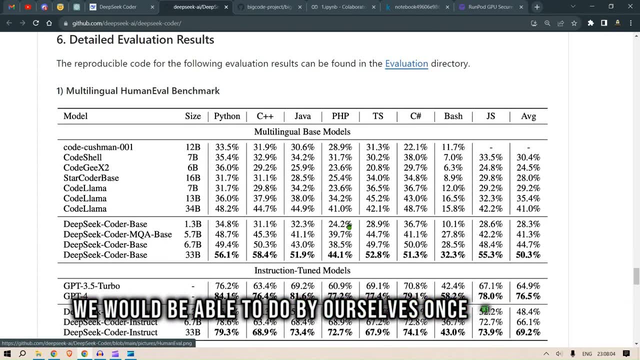 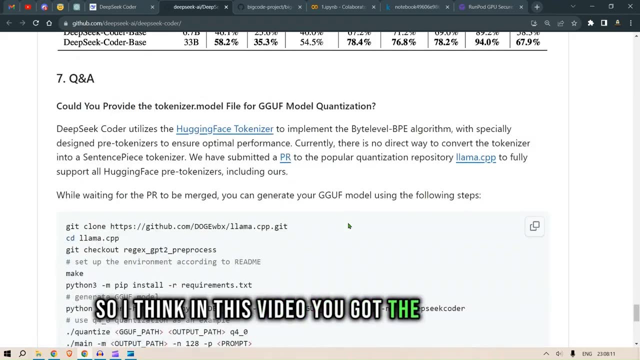 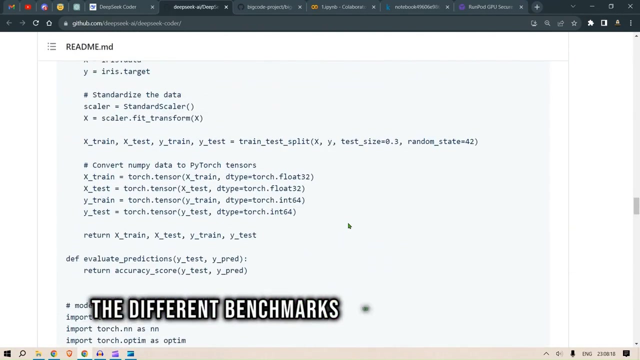 again we need a special format for your own data but this is something uh we would be able to do by ourselves once we create a good model for ourselves so I think in this video you got the basic idea of the different kinds of models or sizes that are available here the different benchmarks that are being tested and for different use cases this model can be used 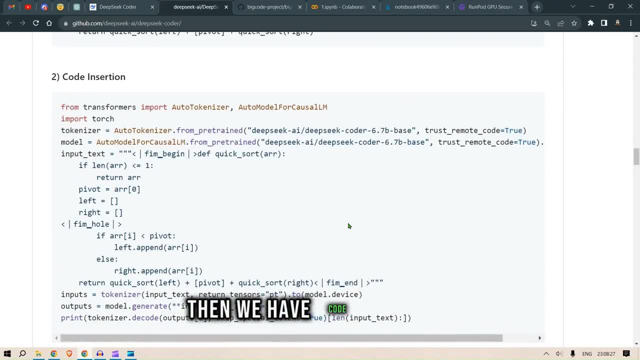 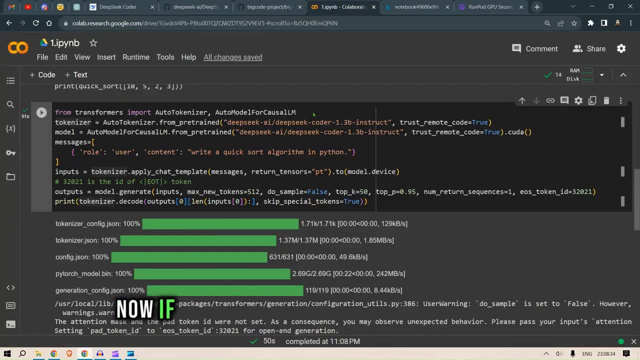 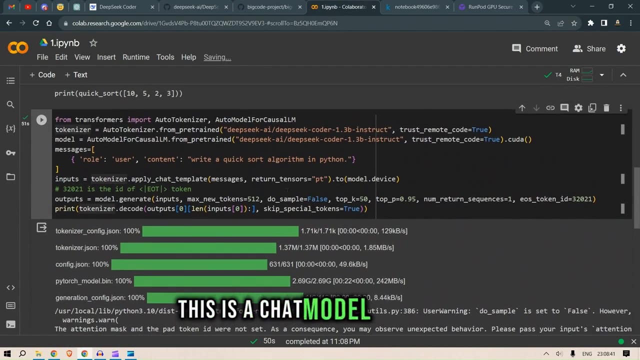 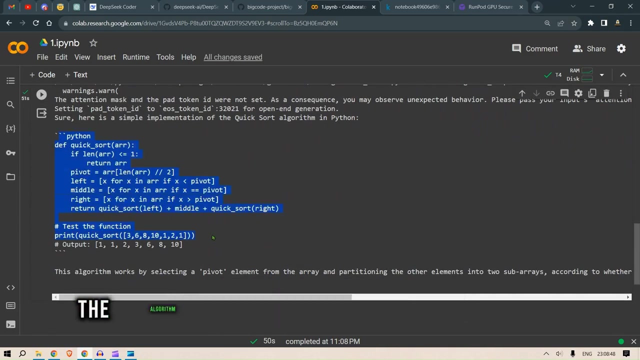 so first is code completion then we have code insertion we have chat model inference we have the repository level code completion now if anything has been completed please let's see this out this was the code this is the chat model inference so that is I think it's pretty good so it gave me the output here the algorithm works by selecting a pivot element from the array and 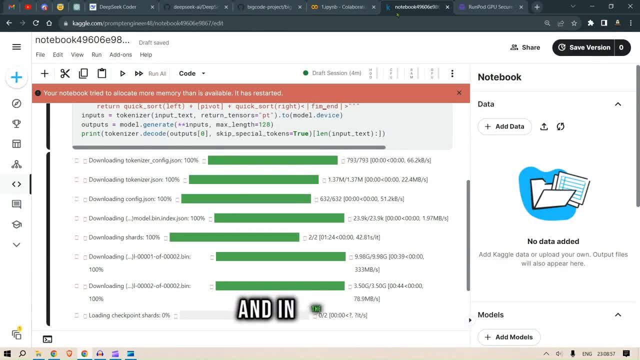 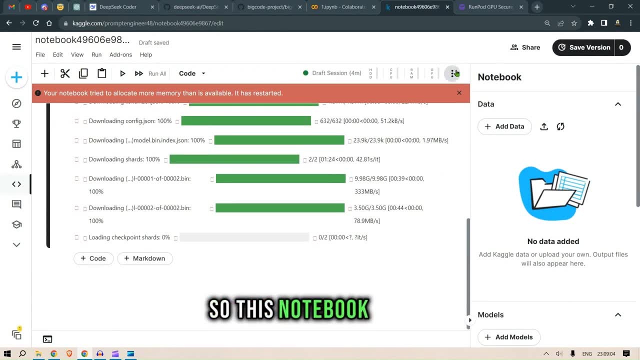 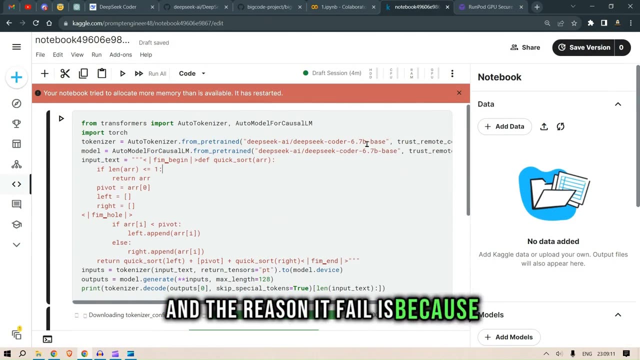 so we have this chat interface like output and in the Kaggle your notebook try to allocate more memory than it's available it has restarted so this notebook failed I'm sorry to say but this notebook failed and the reason it failed is because we have not changed it here 6.7 this 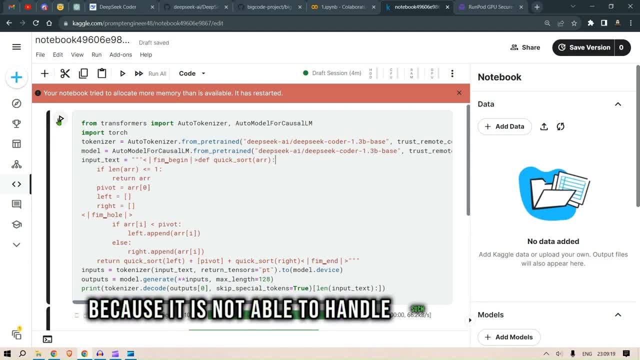 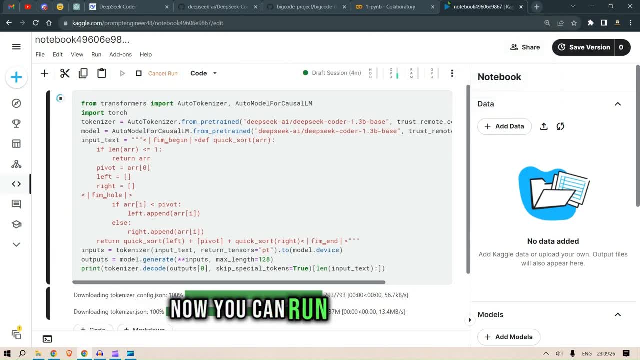 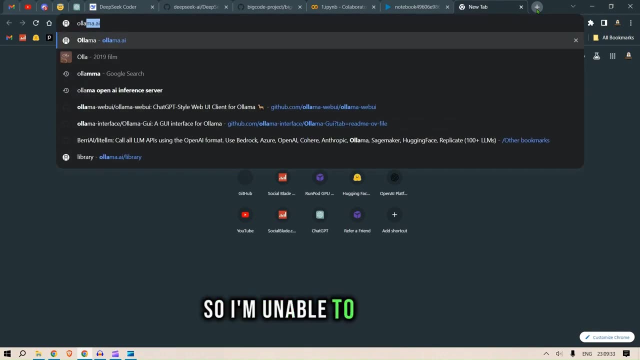 should be 1.3 because it is not able to handle such a big model now again let's run this let's see now you can run this on olama but since I am I'm on my Windows device so I'm unable to run this 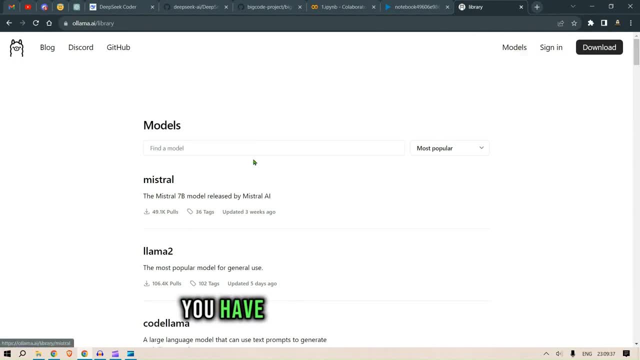 but in the model sections you have the deep seek model a deep seek quarter being added and you can head over to your Mac device and try it try this out using olama I have last two videos dedicated to olama you can use that you can also 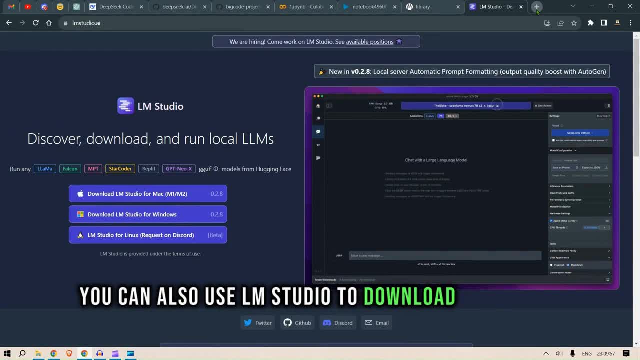 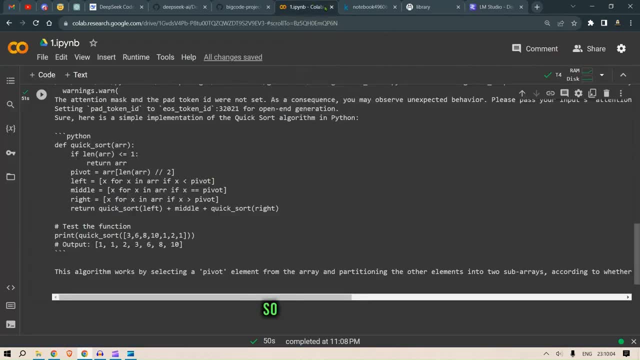 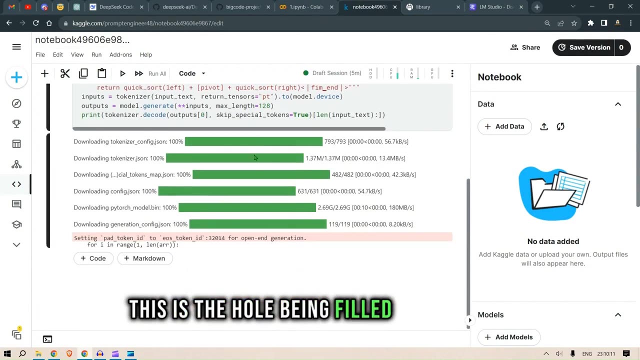 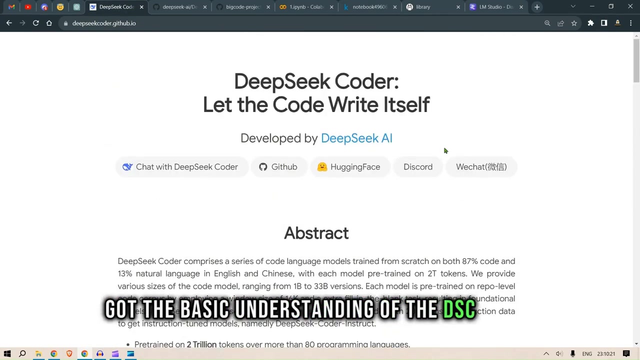 use lm studio to download the model and get your dsc running so let's wait so we can see this output here this is the hole being filled by this code so here we are i think you got the basic understanding of the dsc coder how you can try this out we have different models of four types 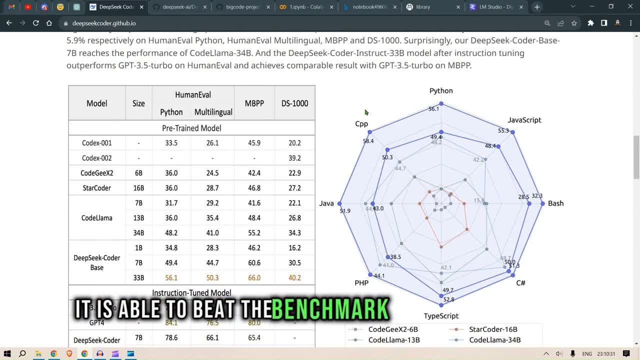 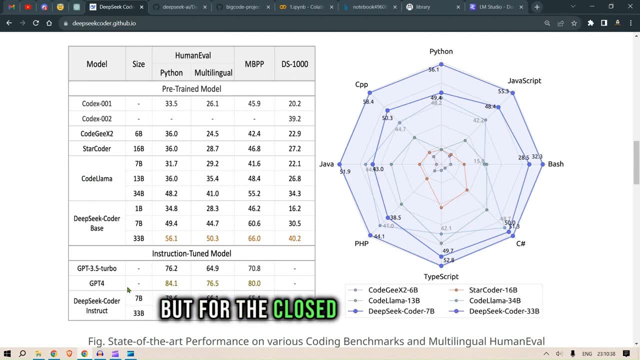 it is able to beat the benchmark of the open source almost all the all the open source models and the pre-trained models but for the closed source models and instruction tune it is able to be at par with gpt 3.5 turbo but it's nothing comparable to gpt 4 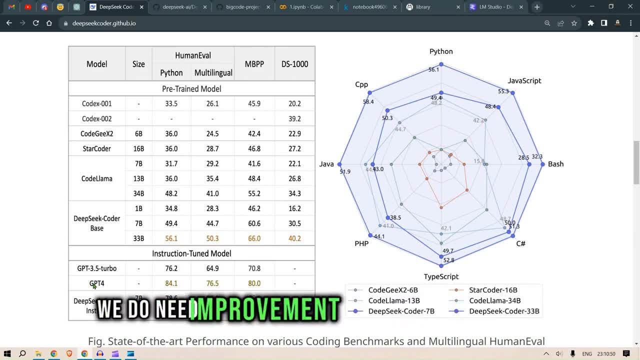 and we do need innovations we do need improvement to get our model to uh at par with gpt 4 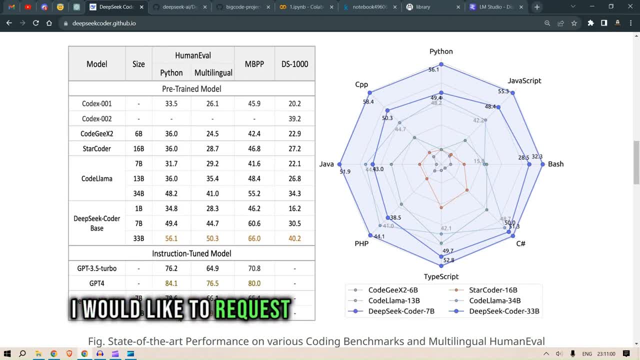 now having said that i would like to request you to go through this paper understand what the authors had in mind 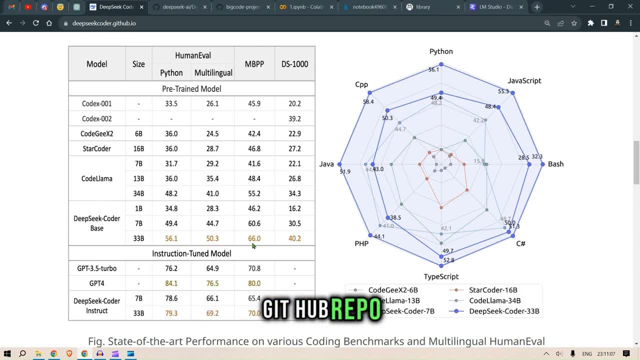 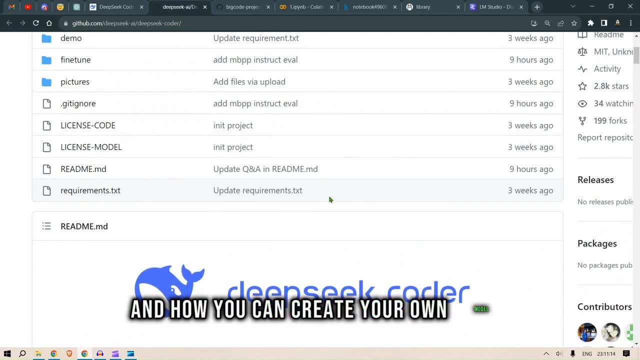 you know go through this github repo understand what the authors had in mind when creating this and how you can create your own model this should be the end of this video and very soon i will 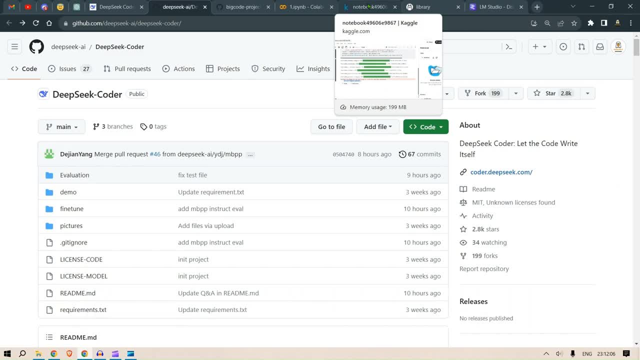 bring out another video on fine tuning of the models because i think this should act as a 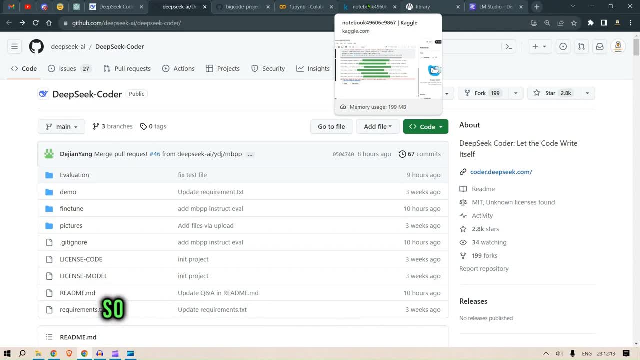 precursor to that the next video so stay tuned for the next set of videos for fine tuning of a model and creating of a model like this at very low cost but since i was out for many days pardon 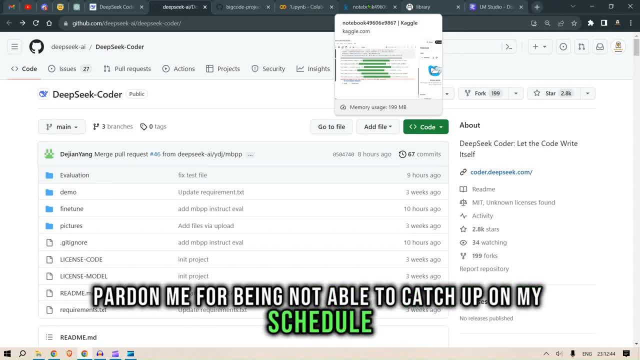 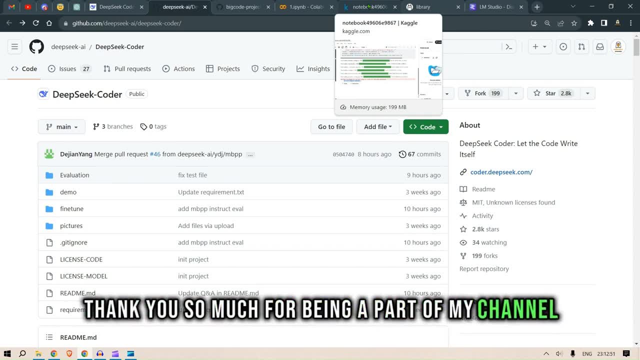 me for being not able to catch up on my schedule but yeah thank you so much for watching thank you so much for being a part of my channel and allowing me to share the knowledge with you 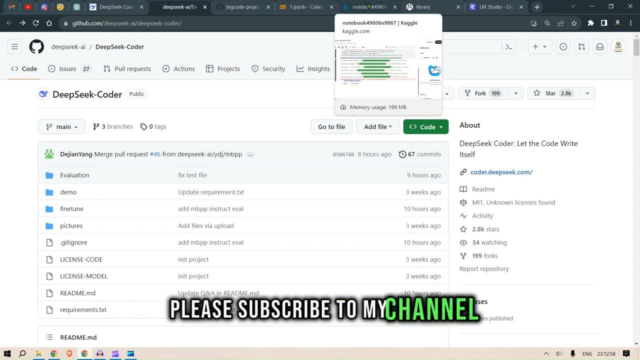 if you like this video please subscribe to my channel like and share this video with your friends and families 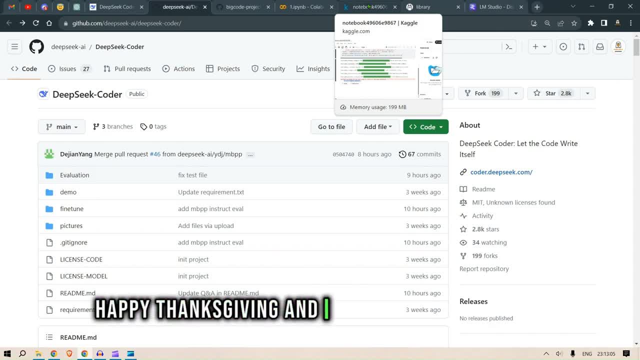 until then happy thanksgiving and i will see you next time please check out the other videos on my channel thank you 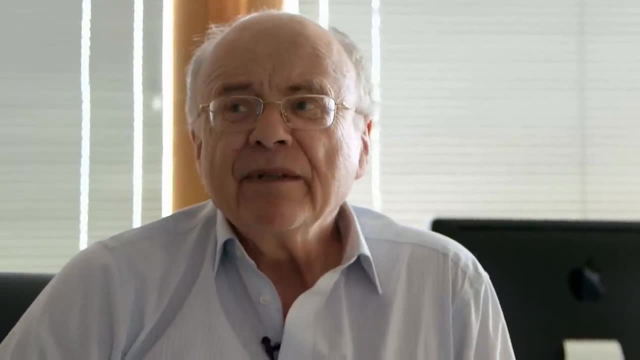 So far we've looked at primitive recursion, Things where you can use recursion if you want to, but you don't have to because it can be de-recursed and turned into an iterative for loop. And we did factorial and we did Fibonacci, both of which are primitive recursive in this sense.